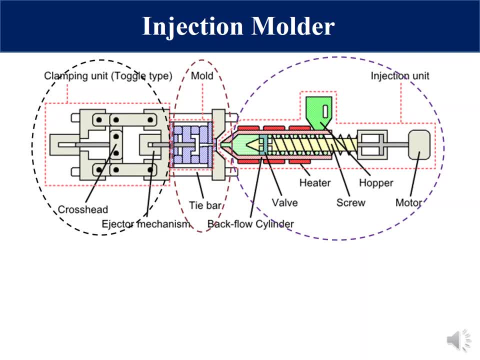 and other. Each of this unit performs a specific task during injection molding cycle. The task of injection unit is melting the polymer and then injecting into the mold cavity. Similarly, the mold performs two main tasks. First one, it provides shape to the product and also 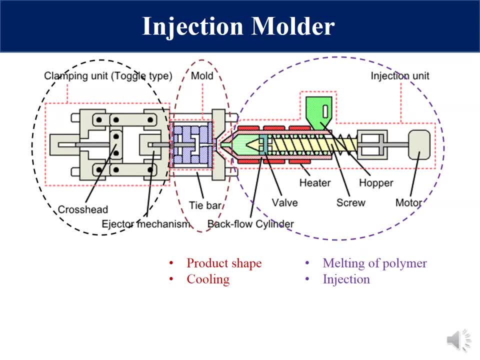 it helps to cool the molten polymer into a solid product. Similarly, clamping unit is responsible for two main tasks. One is called mold mobility. Through this, molds open and closes. And second function is it helps to release the product from the mold. 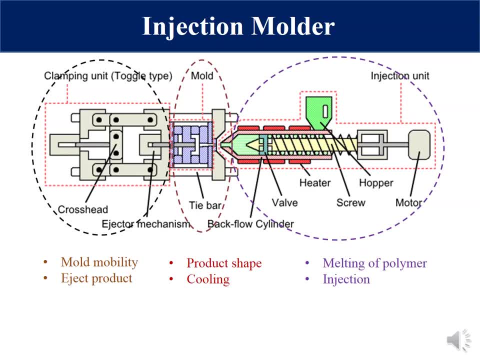 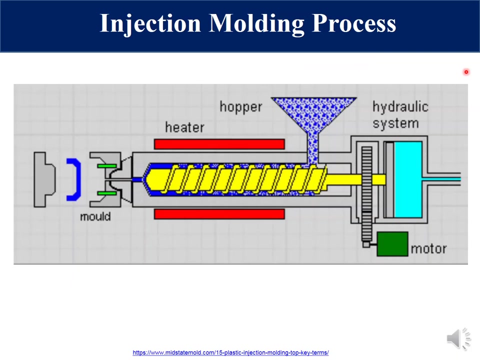 So in injection molding machine, the process by which products are made using injection molding machine is called mold. This is a very important function, because in absence of automatic product release, continuous operation of injection molding is not possible. So let's now discuss about the injection molding process. 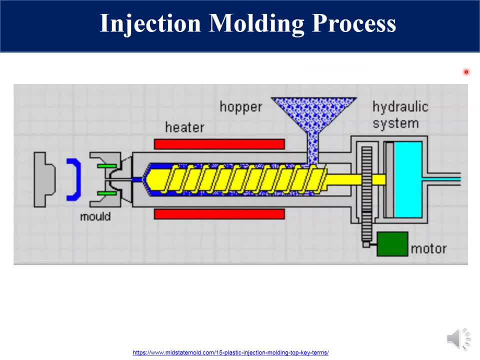 This video is an excellent representation of injection molding process. Here we can see that polymer beads are fed through this hopper and products are coming out of the mold. Now, if we look little bit in more detail how the polymer beads are converted into plastic parts, we can see that polymers are first fed through this hopper, which gets 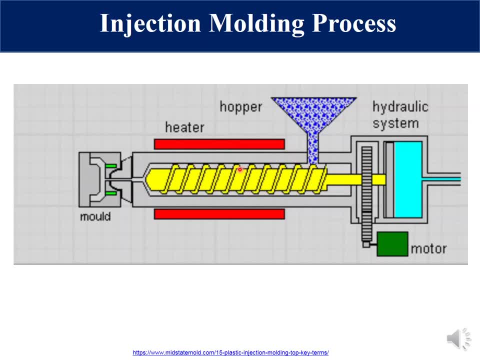 melted inside the extruder, The molten polymer gets is accumulated in the extruder and then in front of the extruder. During this time we can also see that the extruder moves in the backward direction. This mechanism is very similar to the syringe. 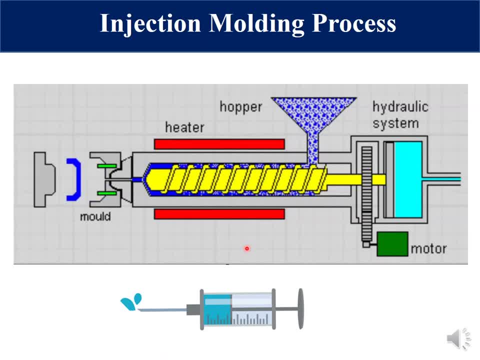 While operating syringe, we have seen that the plunger is moved in the back direction to fill the syringe with the medicine or any other liquid. Then this plunger is pushed forward to inject medicine in our body. Similarly, in case of injection molding, the screw moves in forward direction to inject polymer. 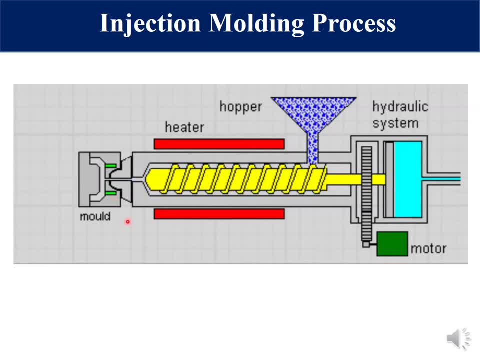 melt in the mold cavity. Now to better understand the injection molding process, we can divide the whole injection molding process in four steps. It will also help us to better understand the injection molding parameters in each step, which controls the whole process and also quality of the product. 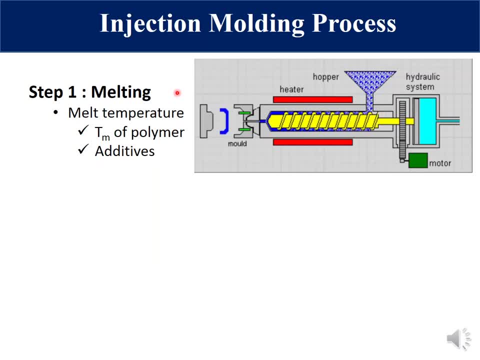 First step is melting. In this step, polymers which are fed through the hopper are stored inside the extruder and stored in front of the screw. The parameter which is very important at this step is melt temperature. Usually extruders are kept at 40 to 50 degrees C higher than the melting temperature of polymer, But the 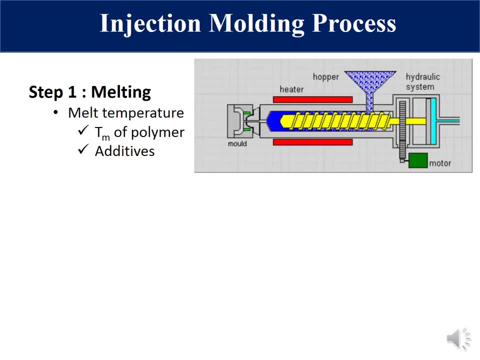 temperature can be lower or higher depending upon the additive present in the extruder, the polymer. if a polymer contains lubricant, the temperature should be lower, otherwise the melt viscosity will be too low. similarly, if the polymer contains nano fillers or reinforcing filler, then the temperature should be higher, so that if the polymer can have sufficient viscosity. 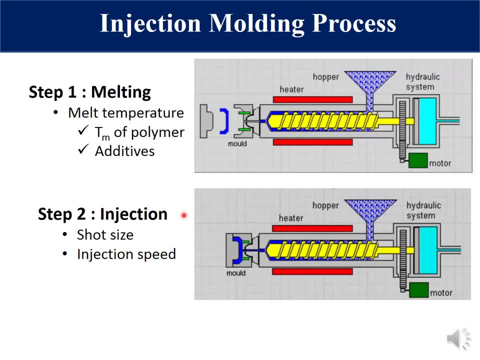 second step is injection. in this step, the screw moves forward and injects polymer inside the mold cavity. now the question is how much polymer need to be injected and second is how fast we need to inject the polymer. so the two parameters- which is very important in this step is short, size, which 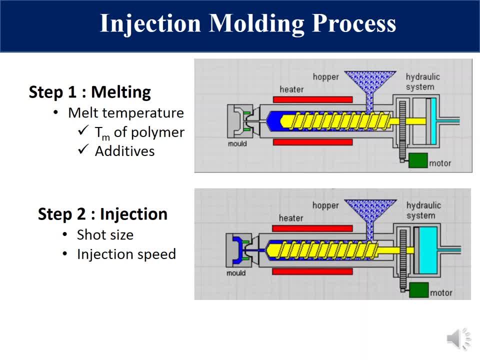 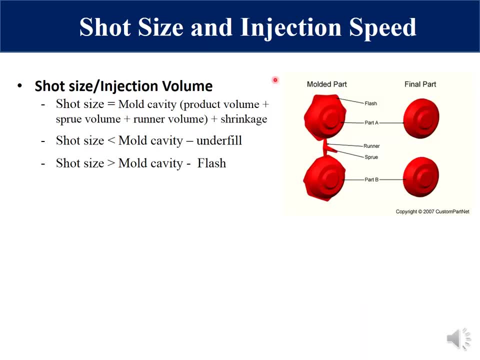 is also called injection time, Injection volume and the injection speed. now let's discuss these two parameters in a little bit more detail. when polymer gets injected in the mold, the polymer need to fill the whole mold cavity, like sprue volume, runner volume, and also the product volume melts when undergoes cooling. 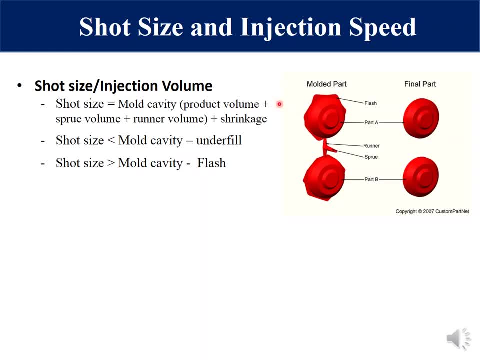 it also leads to shrinkage. so when calculating short size we also need to take polymer shrinkage in the calculation. now two condition may arise. the short size may be smaller than the mold cavity, which is called short short size. this will lead to underfill. second condition is when the short size 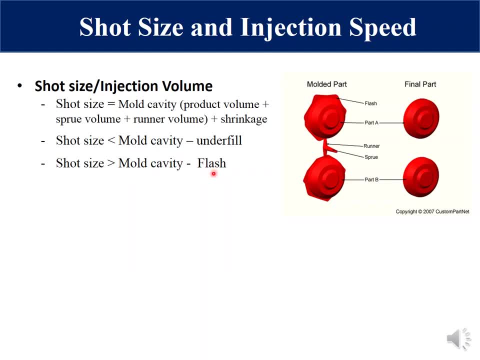 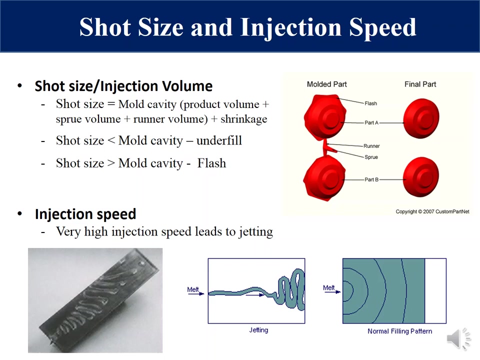 is higher than the mold cavity. in this case flash will occur here. the picture a demonstration of the flash in volume. so the ideal injection volume will be mold cavity plus shrinkage. the next question is how fast we would like to fill the mold cavity. it is always desired to fill the mold as fast as possible. 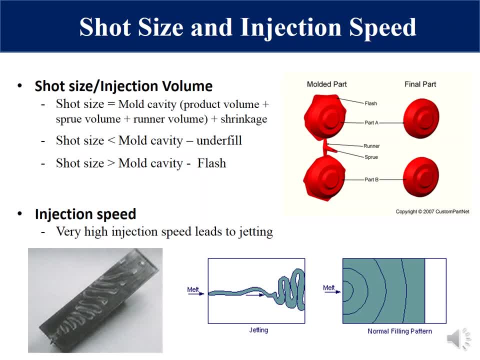 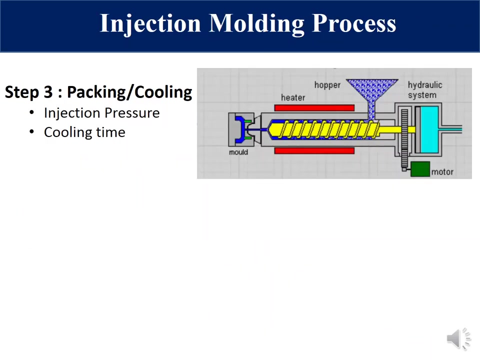 because it leads to higher efficiency of the injection process. But at very high injection speed it leads to jetting which deteriorates the product quality. so the injection speed will be an optimum value between efficiency and the product quality. step in the injection molding process is called packing and cooling. in this step polymer melt. 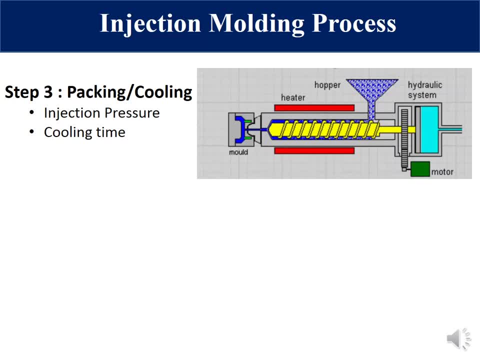 is compressed to get better product uniformity. at the same time, polymer melt is cooled to a solid product. two parameters which are very important in this step are injection pressure and cooling time. higher injection pressure leads to better packing and better uniformity of the product, but injection pressure need to be balanced by the clamping pressure. 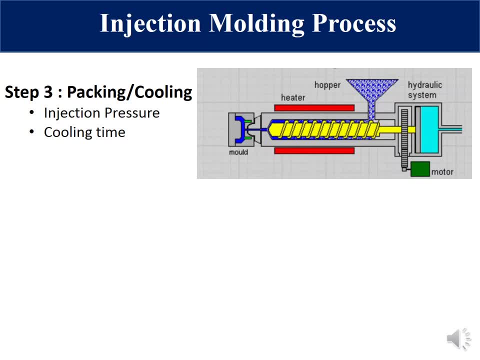 clamping pressure is the pressure between the two mold section. if injection pressure is much higher than the clamping pressure, it will lead to flashing. therefore, injection pressure is decided based on the maximum clamping pressure of the injection molding machine. similarly, cooling time is an optimized value between injection molding efficiency and product. 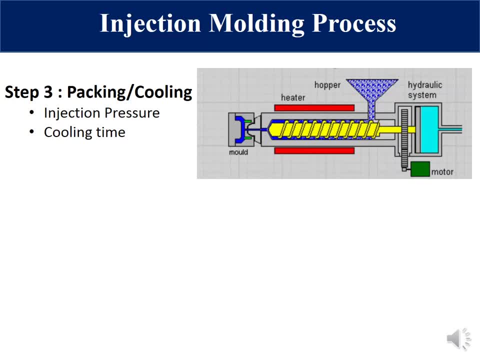 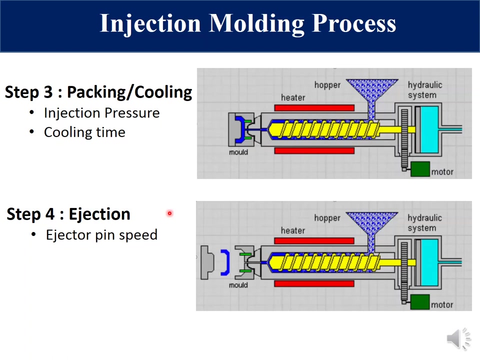 quality. typically, a higher mold temperature leads to product with better strength and gloss, but higher mold temperature requires longer cooling time. so, depending upon the temperature, depending upon the product quality requirement, cooling time is decided, but usually it ranges from 5 seconds to 20 seconds. the fourth step is ejection. in this step, the moving section of the mold moves backward. 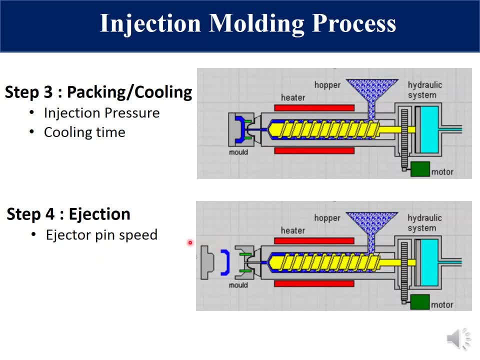 and opens the mold. during this time, the ejector pin pushes the product out of the mold. the product is then collected at the bottom of the machine. in this step, the important parameter is ejector pin speed. a lower speed will be unable to remove the product from the mold. 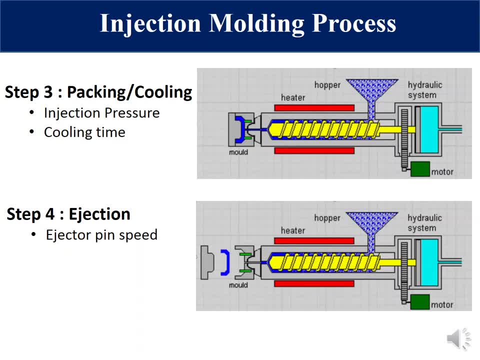 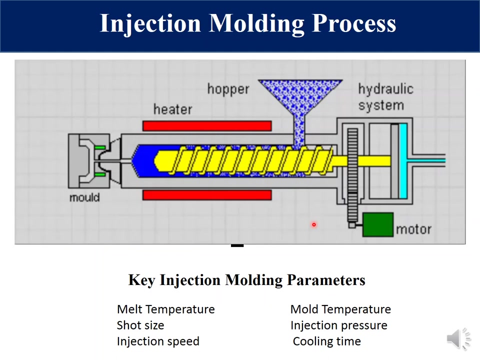 but a higher pin speed will leave a pin mark on the product. so the ejector pin speed is optimized to achieve desired performance and product quality. so during injection molding process, polymer beads are converted into plastic parts in four step melting: injection, cooling and ejection. the key parameters during 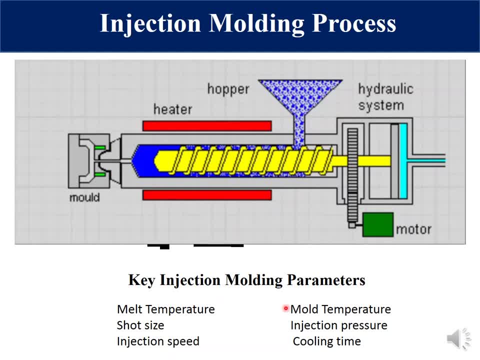 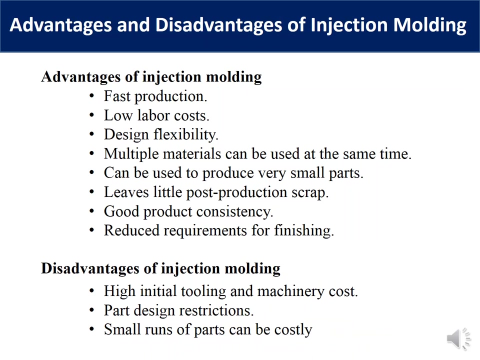 injection molding processes are mill temperature, shot size, injection speed, mold temperature, injection pressure and cooling time. these parameters are highly optimized to achieve continuous production of parts. now let's discuss some of the advantages and disadvantages of injection molding. injection molding is one of the most versatile and efficient product. 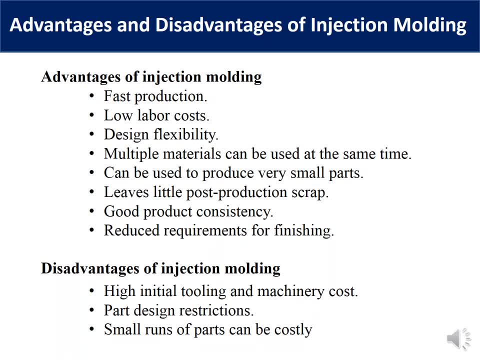 manufacturing process. however, it also suffer from some limitations. some of the advantages and disadvantages of injection molding are listed here. one of the major advantage of injection molding is fast production. once injection molding parameters are optimized, product manufacturing time is only few seconds. another very important benefit of injection molding is low labor cost. 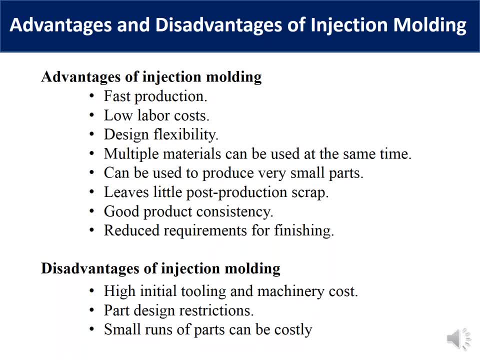 since most of the industrial process are automated, injection molding also offers design flexibility and use of multiple materials. stages of injection molding are: it can be used to produce very small parts. it leaves little scrap and reduces requirement of finishing. because of its automated operation, product quality is very consistent. now, 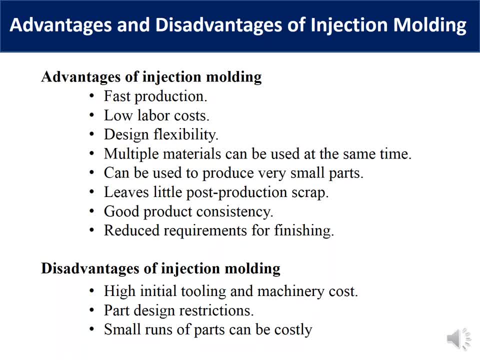 let's talk about some of the disadvantage of injection molding. another critical disadvantage of injection molding is restriction in part design, because shape and size of the part is restricted by the mold size and injection pressure. you should not fulfilling rainfall management with injection molding. injection molding also drink sufficient ride in its design. the other: 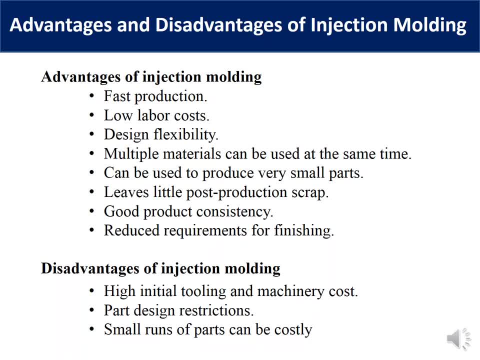 shortage of self- anomalies is amount of sawdust in the machine. injection welding machinesnumber reason that nowadays the injection molding today are at high level price, also in the small run off. injection molding machine is very costly because one of the costly part of the submission 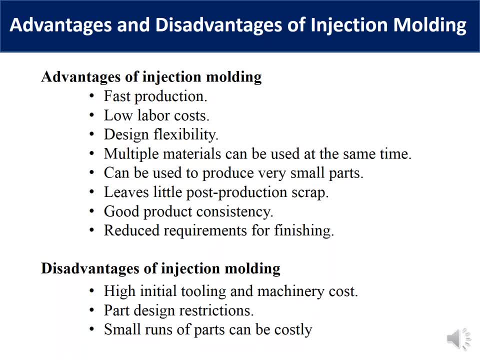 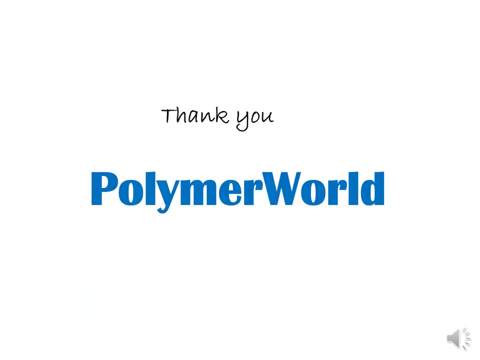 What do you think about injection molding machine? is it mold and one will and disadvantage of injection molding? it become very clear that, whenever possible, it is always advisable to use injection molding for manufacturing plastic products. if you have any question or need further clarification on any section, please comment below. please do encourage us by subscribing to our 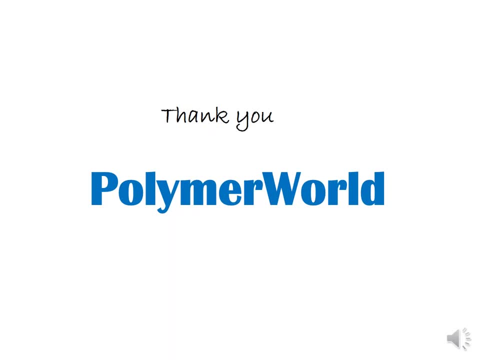 channel polymer world. thank you for watching this video.